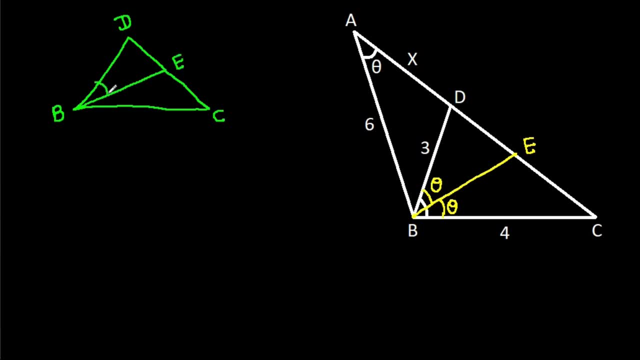 So here in triangle DBC it is DBC over CD. So here in triangle DBC it is DBC over CD. BE is angle bisector, so BD over BC. it will be DE over CE and BD is 3, and BC is 4.. 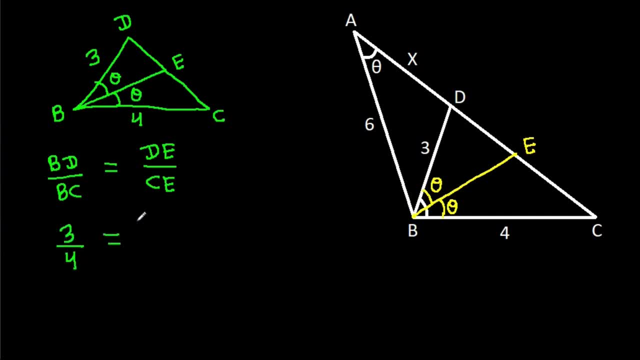 So it is 3 over 4 is equal to DE over CE. That is all means if DE is 3A, then CE, it will be 4A. If DE is 3A, then CE, it will be 4A. 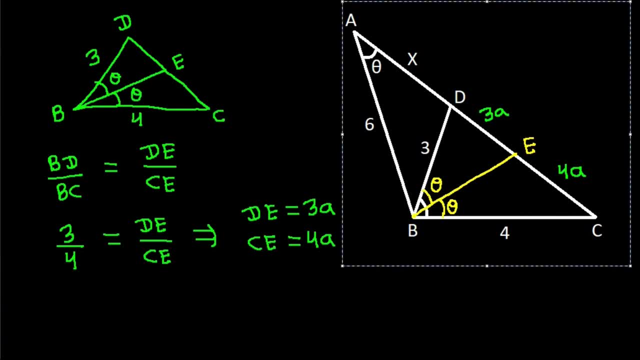 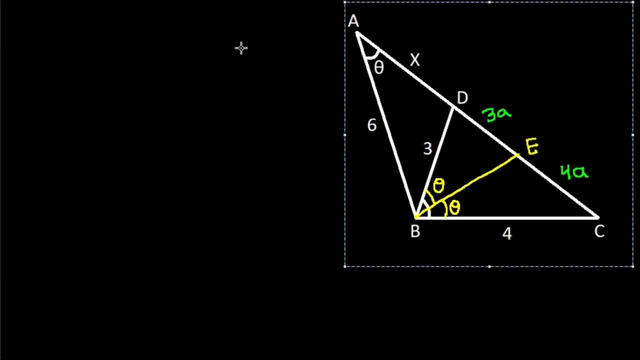 Now in triangle AEB and triangle BED we have: angle AEB is equal to angle BED, that is common. and angle EAB it is equal to angle EBD, that is theta. So the angle is equal to angle EBD, that is theta. So the angle EBD, that is theta. So the angle. 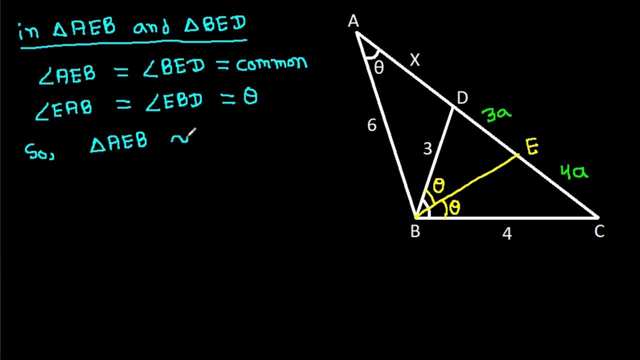 AEB. it will be similar to triangle BED. Hence AE over BE it will be equal to. EB over ED. it will be equal to AB over BD And AE. it will be x plus 3A. AE is x plus 3A over BE. it is equal to and EB it is. BE over ED. it is 3A. 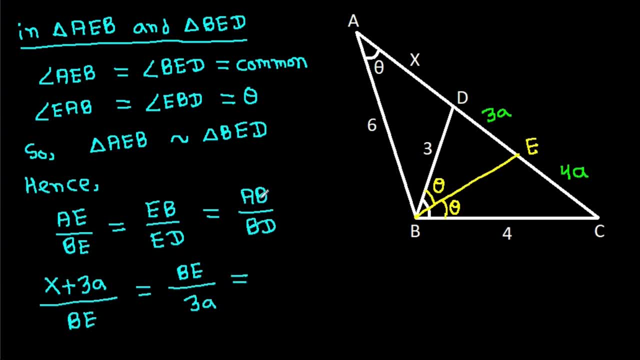 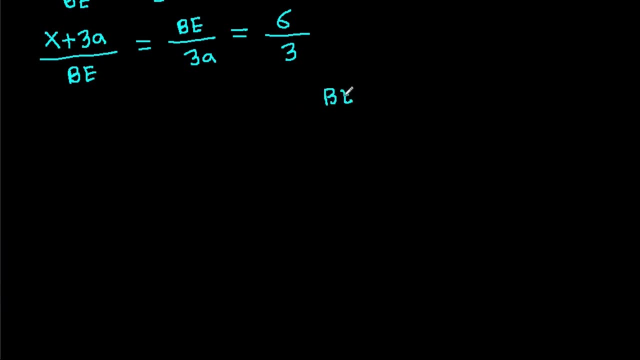 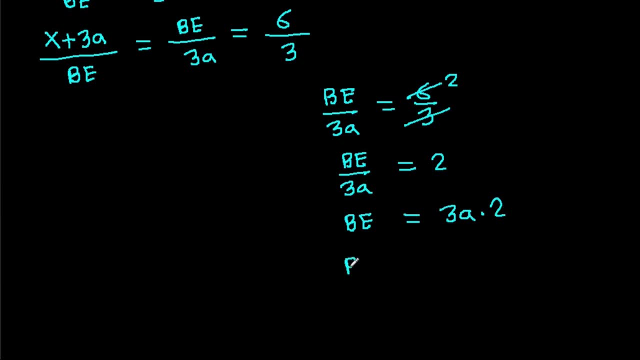 it will be 3A times 2, so BE it will be 6A, and we have X plus 3A over BE. it is 6 over 3 and 6 over 3 it is 2. so X plus 3A it will be 2 times BE. 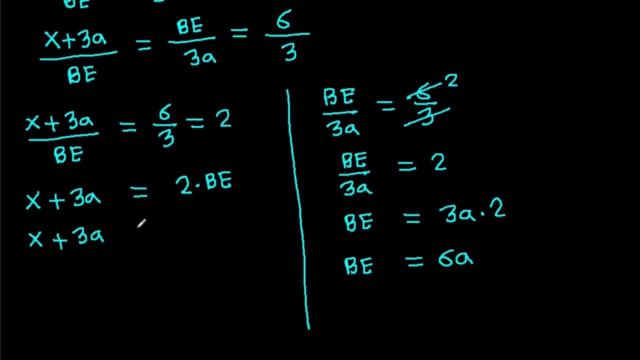 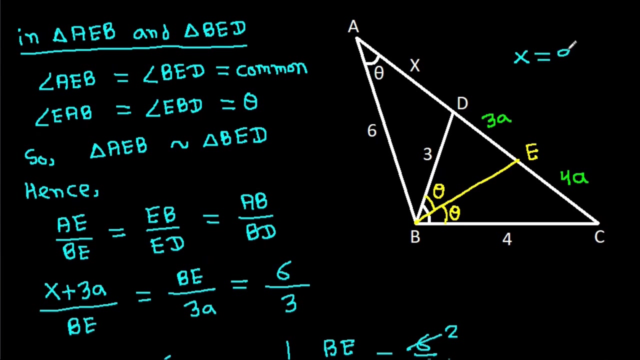 And x plus 3a, it is equal to 2 times and be it is 6a. be is 6a. So x plus 3a it is 12a. So x will be equal to 12a minus 3a, So x it will be 9a. We get x is 9a and 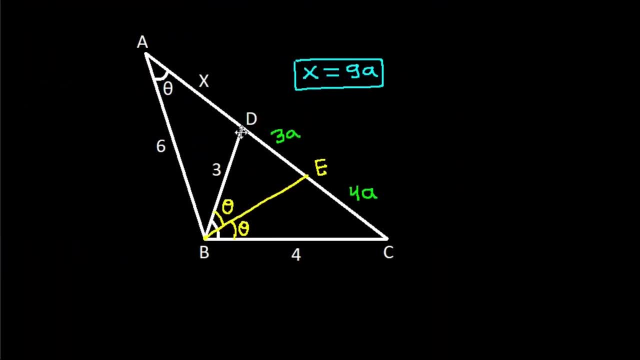 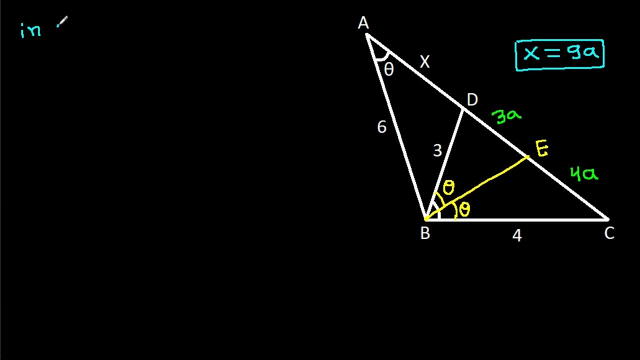 be. it is 9a Now in triangle ACB and triangle BCE angle ACB. it will be equal to angle BCE Now in triangle ACB and triangle BCE angle ACB. it will be equal to angle BCE Now in. 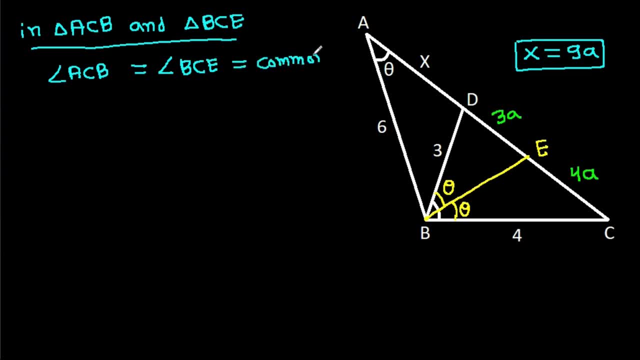 triangle ACB and triangle BCE. that is common. And angle CAB it will be equal to angle CBE. that is theta. So triangle ACB- it will be similar to triangle BCE Now in triangle ACB and triangle ACDB. circle ACB will be similar to triangle ACB and angle. 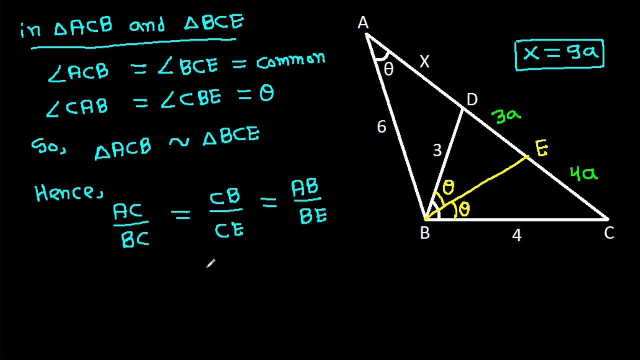 aze will be equal to angle A, E, corresponding to angle uf or uf comma. Now in triangle 20 Guessing duration will be similar to angle 80. Then we also have that angle ACB, and angle plus 7a over bc is 4, it is equal to cb. it is 4 over ce, is 4a, it is equal to ab, is 6 over be. 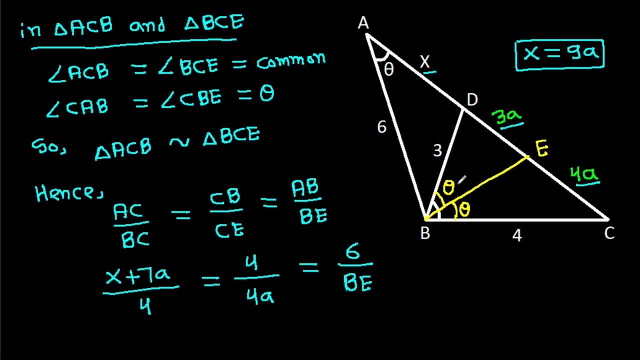 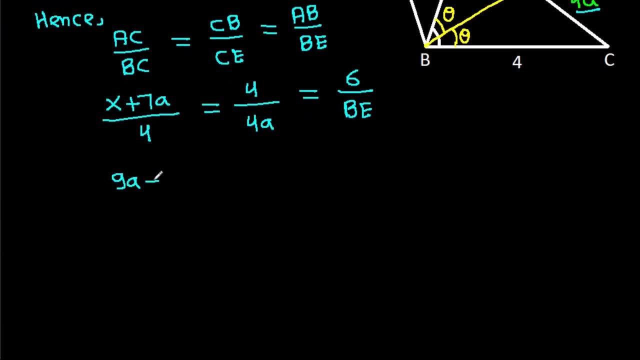 and we have x is 9a, so x is 9a plus 7a over 4, it is 4 over 4a and 4 will get cancelled and it is 16a over 4 is equal to 1 over a. 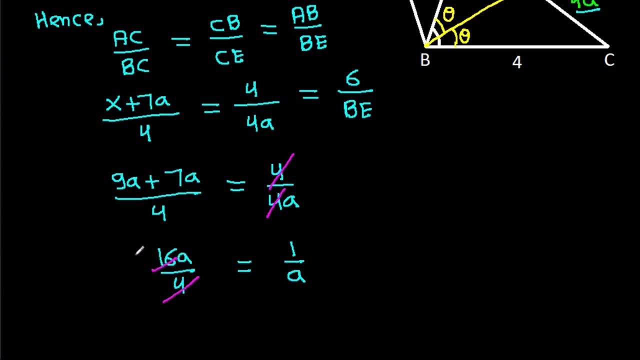 and we have x is 9a plus 7a over 4. it is 4 over 4a. and we have x is 9a plus 7a over 4. it is equal to 1 over a, and 4 times 4 is 16. 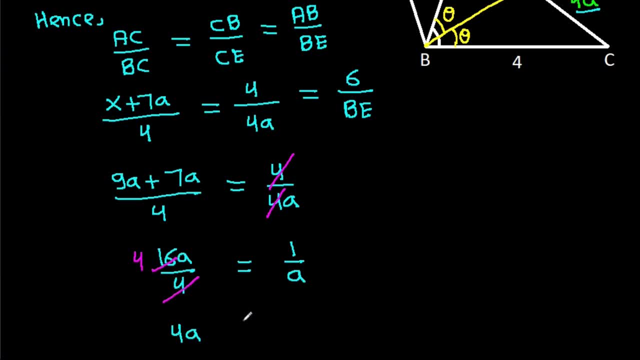 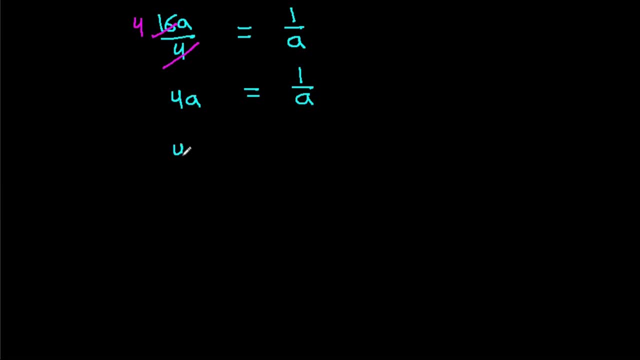 so 4a it is 1 over a and 4a times a it will be 1 and 4a. square it is 1, so a square it will be 1 over 4 and a it is 1 over 4 and a it will be plus, minus root under 1 over 4.